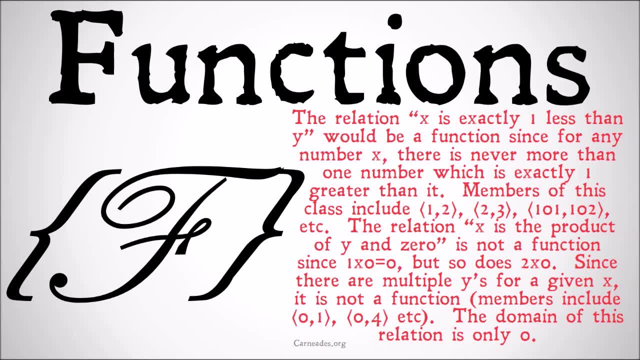 since for any number x, there's never more than one number which is exactly one greater than it. Members of this class would include 1, 2, 2, 3, 101, 102, etc. The relation x is the product of y and zero is not a function, since one times zero equals zero, but so does two. 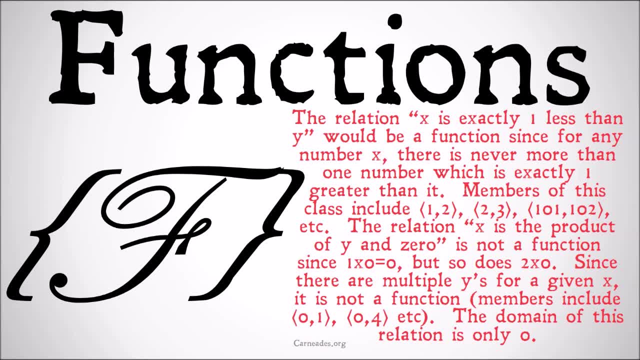 times zero. There are many y's which fit with the same x. Since there are multiple y's for a given x, it is not a function. Members of the relation would include 0,, 1,, 0,, 4,, etc. The domain of this. 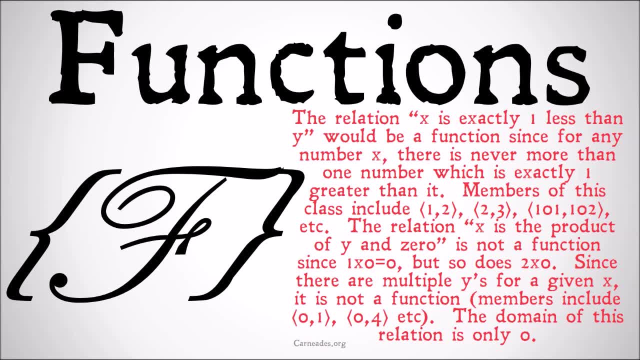 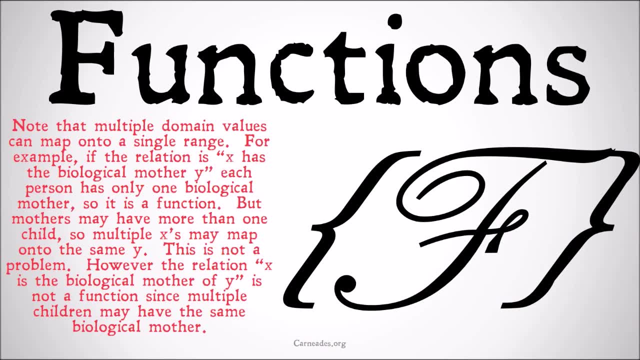 relation is only zero, but it has a wide ranging range and so it's not a function. Note that multiple main values can map onto a single range. For example, if the relation is, x has the biological mother y. each person has only one biological mother, so it is a function, But mothers may have. 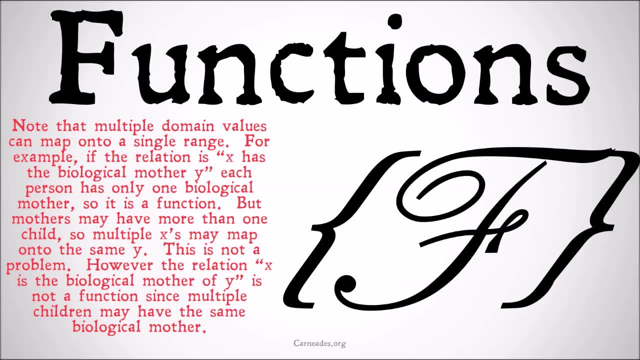 more than one child. so multiple x's may map onto the same y. This is not a problem. However, the relation x is the product of y. However, the relation x is the biological mother of y is not a function, since multiple children may have the same biological mother. So, to be clear, where x is the child having a mother and 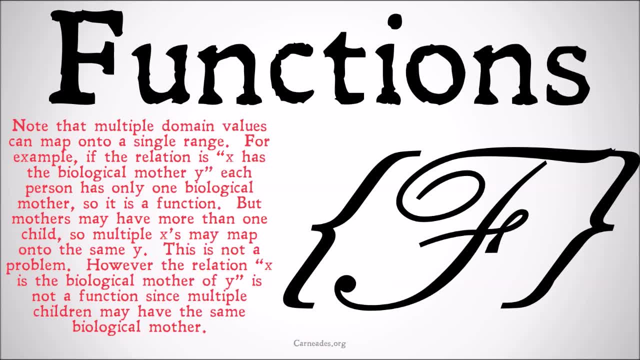 multiple children can have the same mother and the child is the in the domain, the first half of the relation. it's fine to be a function, But when x is the mother, since that can map onto multiple people, the domain is a single person but the range has multiple options for. 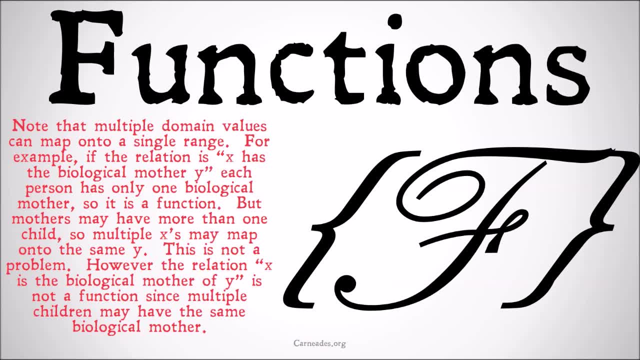 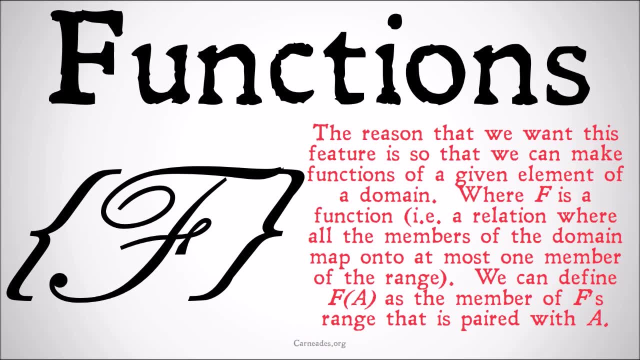 each individual person. that's not a function, and we'll see why in just a second. The reason that we want this feature is so that we make can make functions of a element of a domain where f is a function, ie a relation where all members of the domain map onto, at most one member of the range. 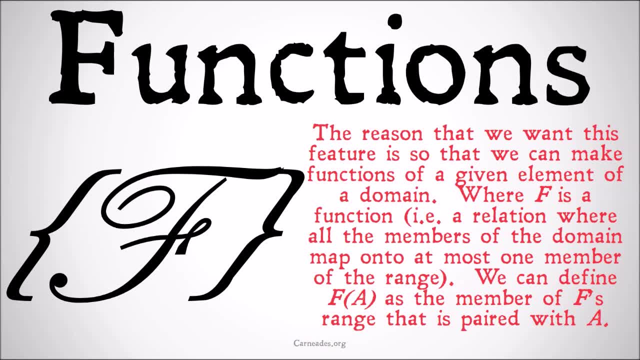 We can define f as a function of a domain and we can also map onto at most one member of the range. We can define f of a as the member of f's range that is paired with a, and there's always only going to be one value that that spits out It might be the same value as something else. you 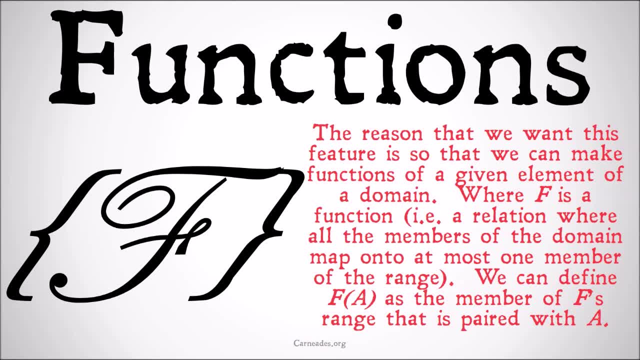 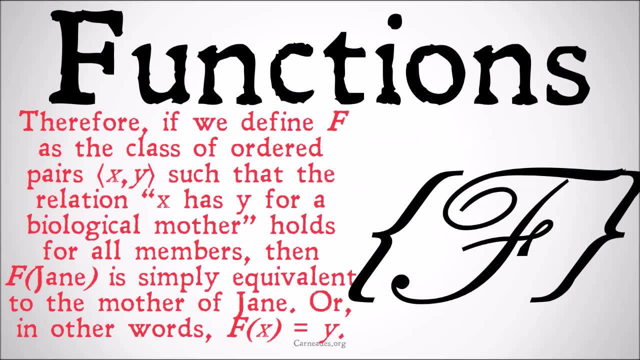 put into that function, but there's always only going to be one value that gets spit out of that, So it's always defined as just one thing. Therefore, if we define f as the class of ordered pairs- x, y- such that the relation x has y for a biological mother holds, 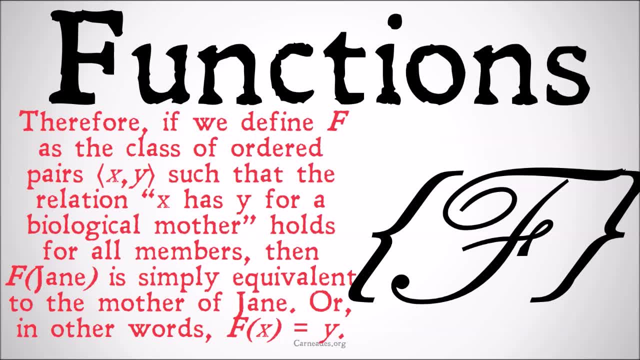 for all members, then f of jane is simply equivalent to the mother of jane. It identifies one individual. but if we had switched that around, jane's mother might have multiple children, and so the child of someone isn't going to be a function because it maps on to multiple people or in other. 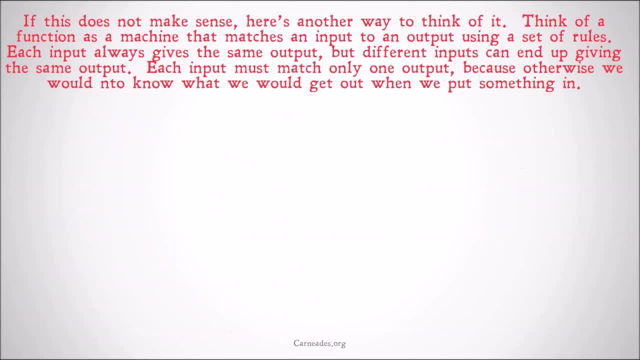 words f of x equals y. So if this doesn't make sense, here's another way to think of it. Think of it like this: Our function is the machine, the class of the ordered pair a, b, the ordered pair 1- 10,. 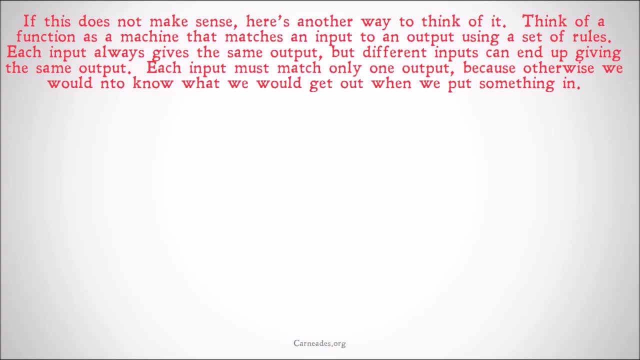 the ordered pair red, blue and the ordered pair 3.. So we can see that the function is the machine that matches an input to an output using a set of rules. Each input always gives the same output, but different inputs can end up giving the same output. Each input must match only one output. 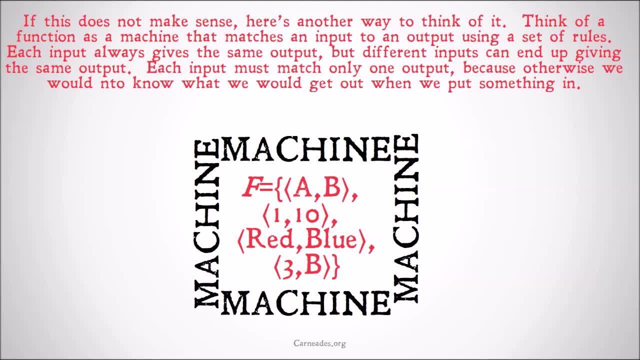 because otherwise we would not know what we're going to get when we put something in and we always follow kind of the same rational set of rules. So think of it like this: Our function is the machine, the class of the ordered pair, 3, b. When I put a into this machine, I get out b, because the function 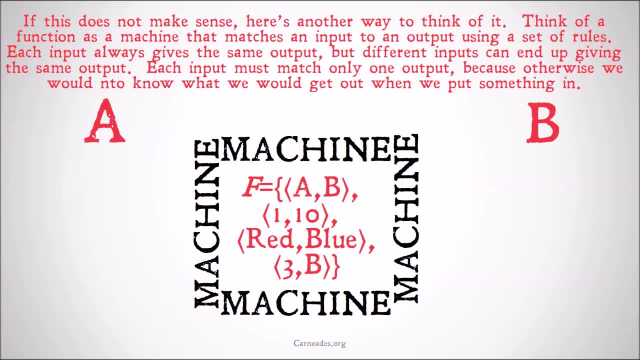 of a. the value a is paired with is b, So the function of a is b. When I put 1 into the machine, I get out 10, because the function of 1 is 10 or the value that is paired with 1 in the ordered. 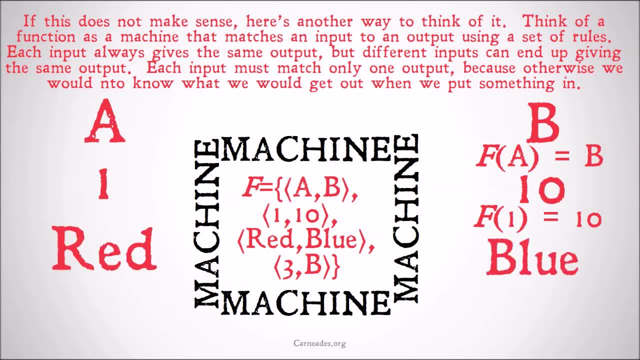 pair within the function is 10.. When I put red into the machine, I get out blue because f of red b is b. And when I put 3 into the machine, I get out b because f of 3 is b. Hopefully this is clear. 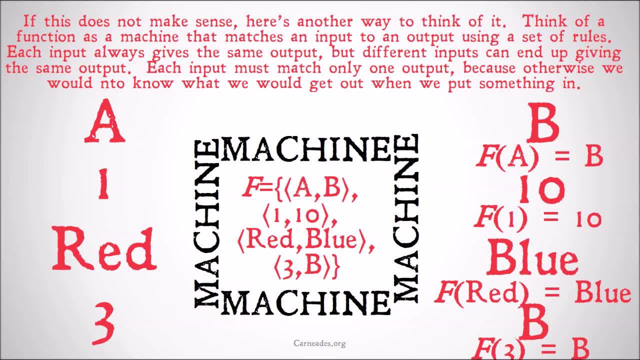 why the inputs, the domain, can only match with one range. because if I had two values that a matched with, then I wouldn't know when I put the a into the machine what would be spit out. We use several terms when speaking about functions. If the domain of a function 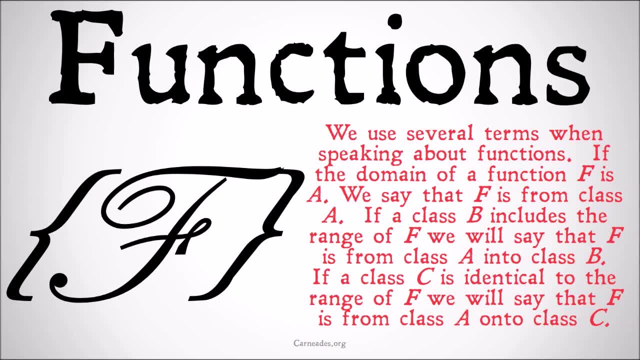 f is a, we say that f is from class a. If a class b includes the function a, we say that the function f is from class a. the range of F: we will say that F is from class A into class B. If class C is identical with the. 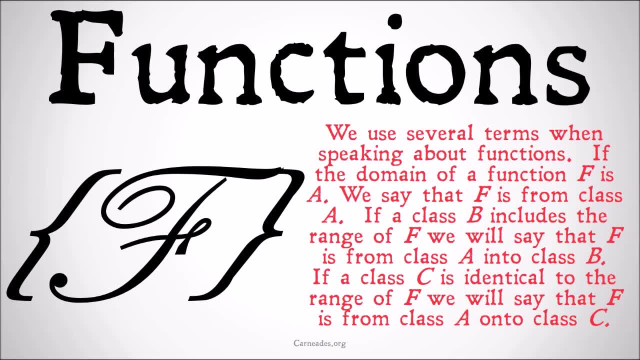 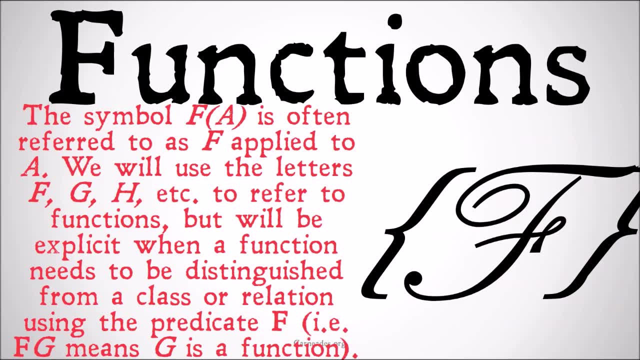 range of F. we would say that F is from class A onto class C, And we're going to get into more of this. when we talk about injection, surjection and bijection, The symbol F of A is often referred to as F applied to A. We'll generally use the letters F, G, H, etc. to refer to functions. 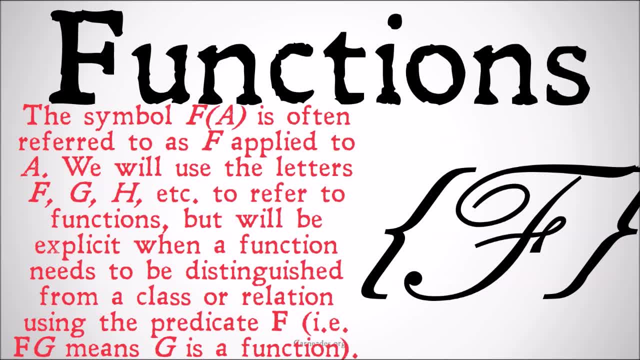 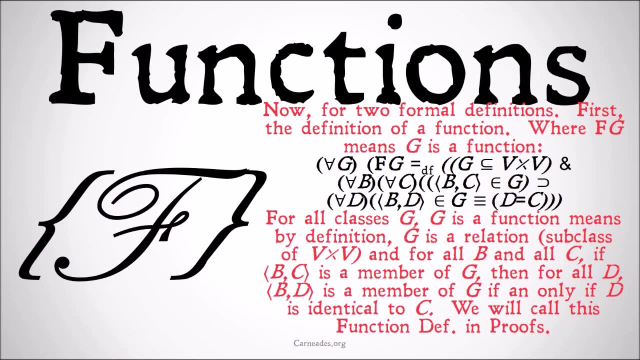 but we'll be explicit when we're using a function, when using a function needs to be distinguished from a class or relation. Using the predicate F, ie FG means that G is a function. Now for two formal definitions. First, the definition of a function where F of G means 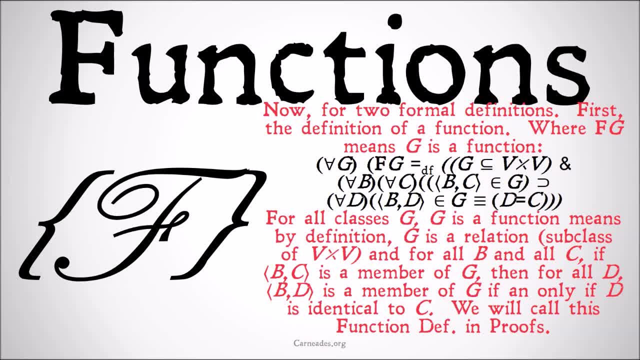 that G is a function. So for all G, for all classes, G G is a function means by definition that G is a subclass of the universal Cartesian product or the Cartesian product of the universal class in itself. and for all b and all c, bc is a member of g. 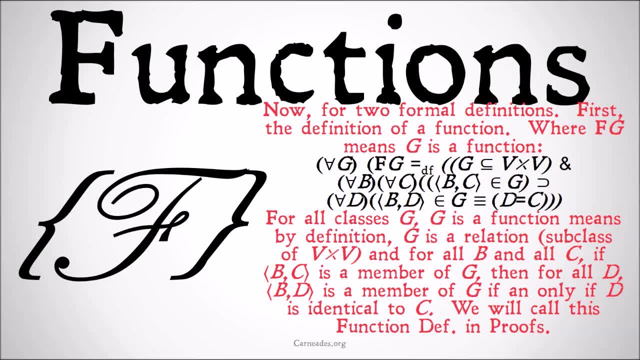 implies that for all d, bd is a member of, g is materially equivalent to d is equal to c. So, basically, what we're saying is for all pairs of ordered, for all ordered pairs that are members of g if they're for the range. 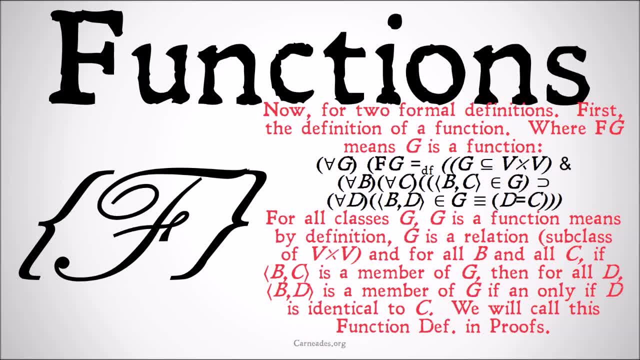 there's only one value for the range. For the range for all of those c that could possibly fit after b, for all d that also fit after b. they're. all those d are identical to that original c. Hopefully that makes some sense. 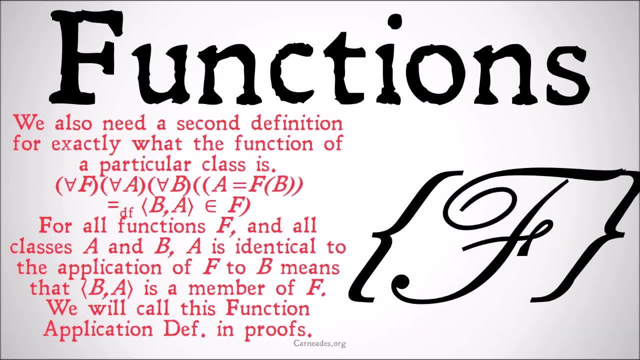 We're gonna call this function definition. in proofs, We also need a second definition for exactly what a function of a particular class is. We're gonna use: call this for all: f for all, a for all b. a is equal to f of b. 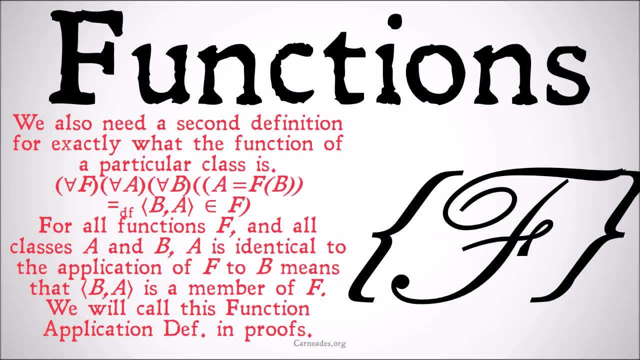 means by definition that b a is a member of f. So if we want to say f of b equals a, where the function applied, function f applied to b is a, that means that one of the members of f is the ordered pair b a. 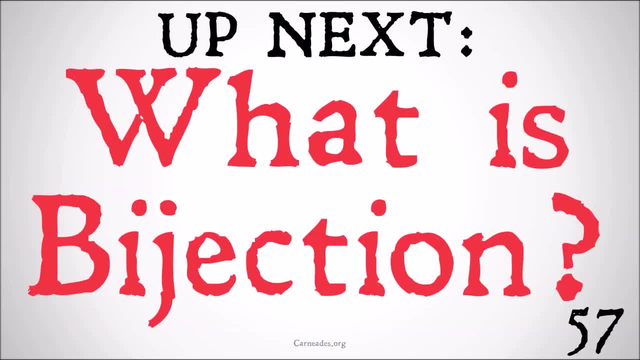 We'll call this function application definition in proofs. Whew, that was a good one Up. next, we'll look at what is bijection. Stay tuned for a brand new video every single day for the whole month of October, here with carneadesorg. 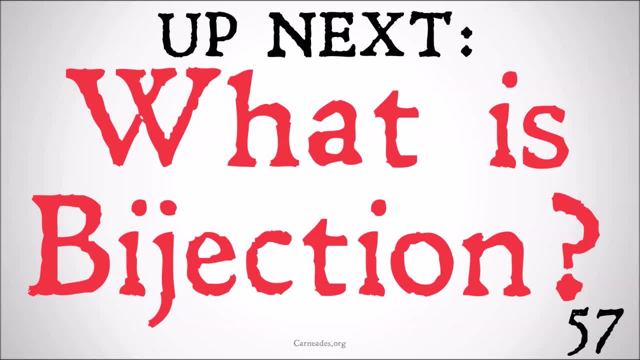 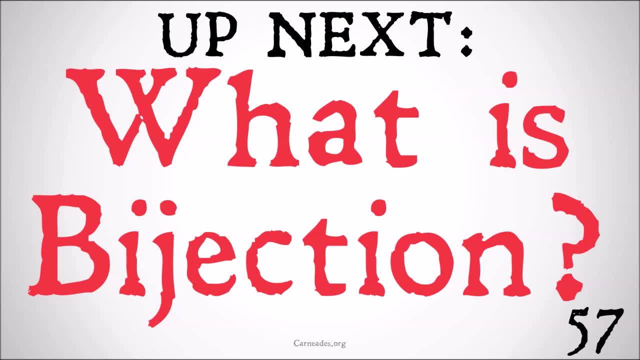 stay up on these videos And if you like this content and want to make sure you don't miss any of the six months of set theory, watch this video and more here at carneadesorg and stay skeptical, everybody. 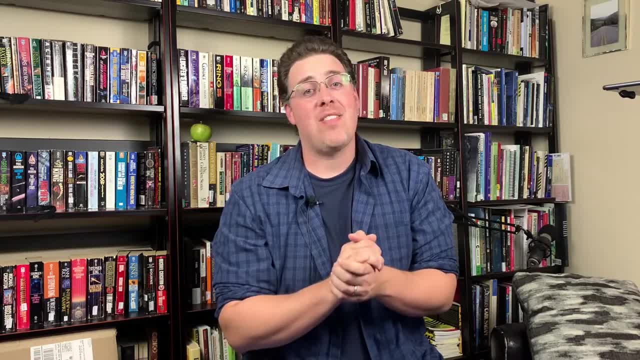 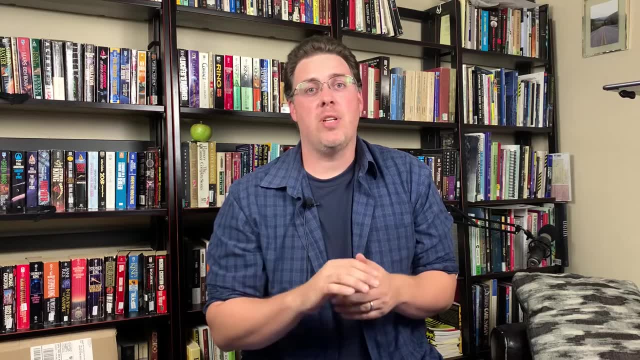 Hello and welcome to Homeschool Together. Today we are going to be reviewing the mathematical reasoning Lettable A Kinder Curriculum. Now. we've done a longer podcast on this and it's in the show notes below, but today we're going to be doing a little bit of a walkthrough, Just a. 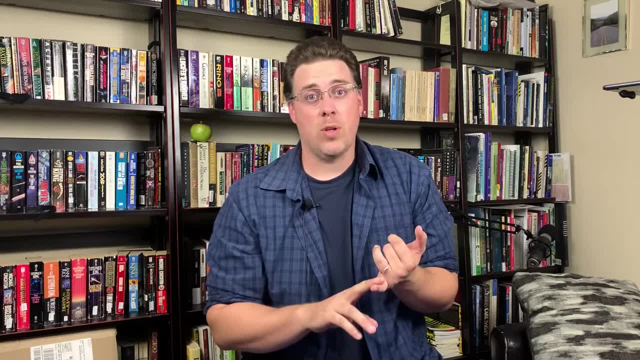 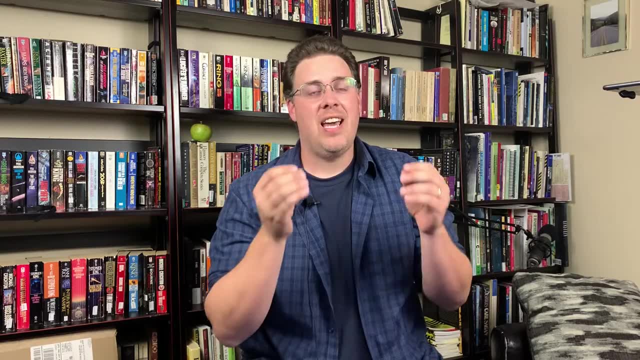 couple pieces of information on this curriculum. It is an all-in-one workbook. It is aligned to the National Council of Teachers of Mathematics, which is Common Core. aligned, It's $30 and it follows a spiral method where we turn back and back and back again on common concepts, as you 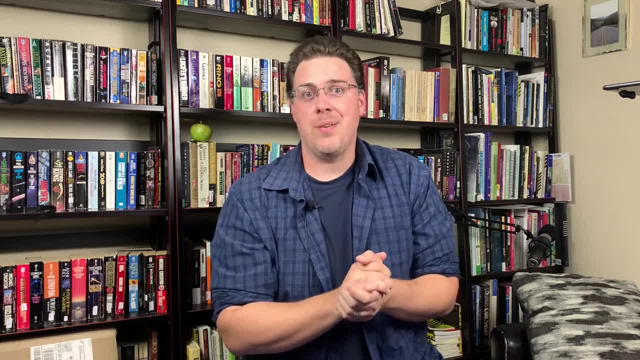 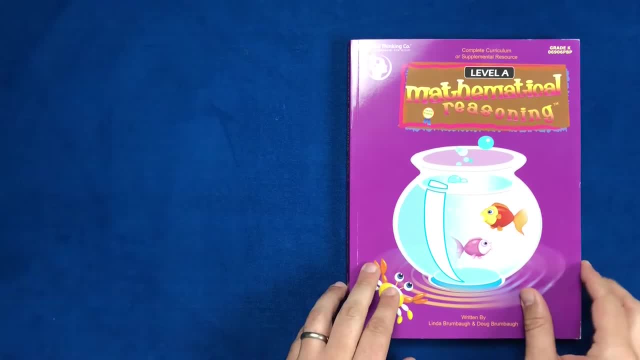 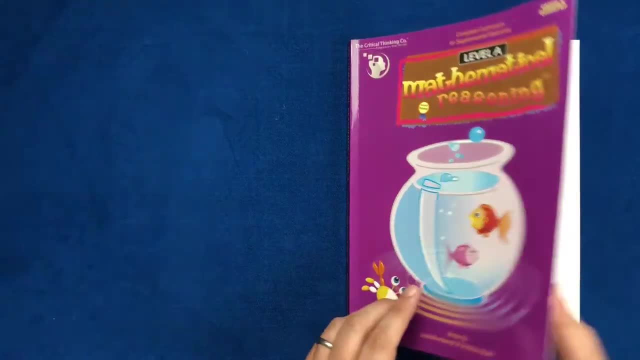 move through it. So let's hop into it and take a look at this curriculum So, as we can see, nice little workbook, pretty drawings and colors, very colorful Indicates level A. so make sure you get the right curriculum when you're looking on the Critical Thinking Company's website. So